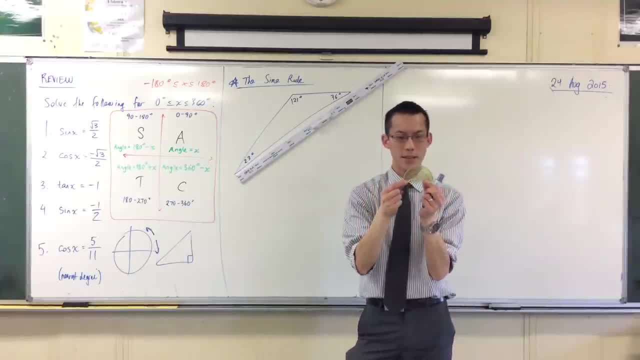 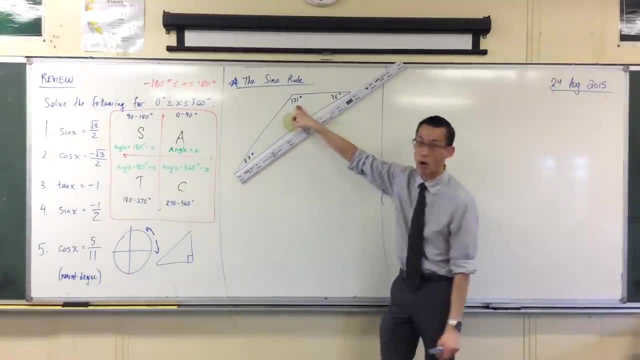 So, for instance, the closest that this thing can measure is a whole degree, right, That's what all the markings are: 180 degrees all the way around here. So if you've got an angle that's not exactly a whole number, then you're forced to approximate, right. 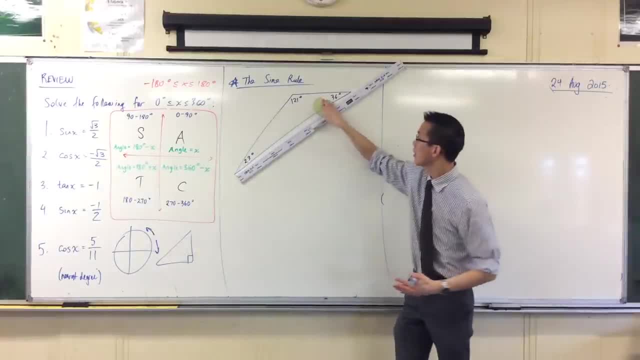 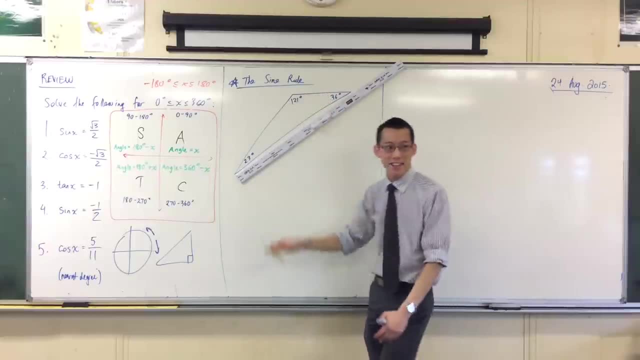 You might approximate up, you might approximate down. Now, if there are a couple of angles and you approximate both of them up, Because, Because, Because- it's like, oh, that's the closest thing- When you add them, you're going to get more than 180 degrees because you've approximated upward. okay, 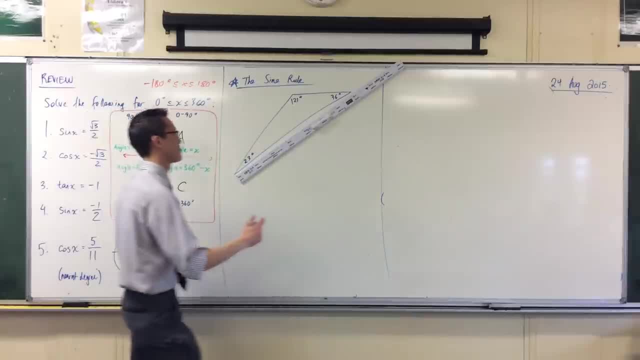 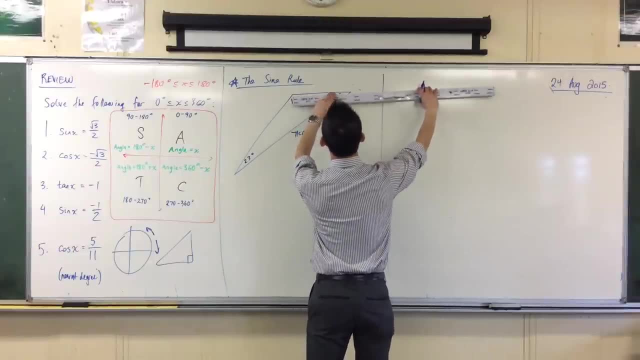 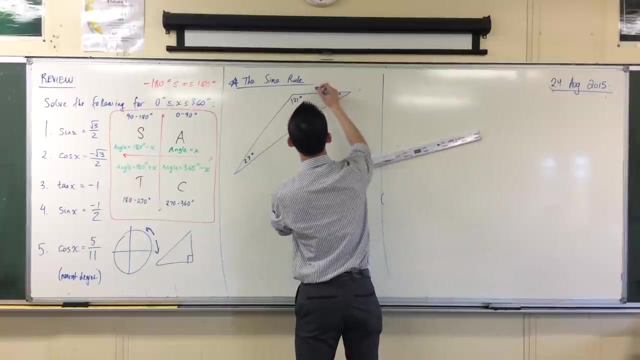 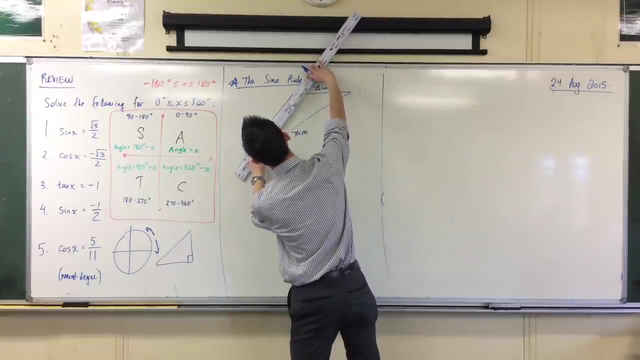 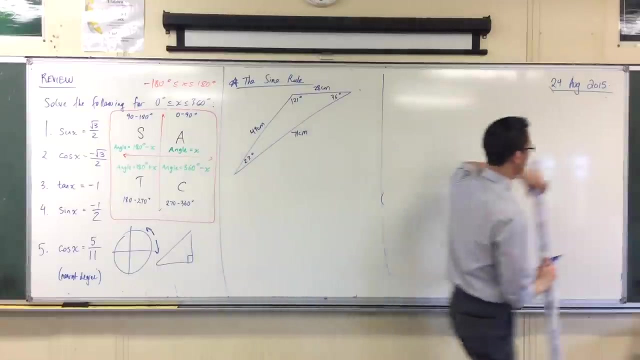 So it's okay. That's kind of just what happens. Don't forget the distances, Don't forget the angles. Don't forget the angles, Don't forget the angles. Can you give me a show of hands if you've done all your angles on all your sides? 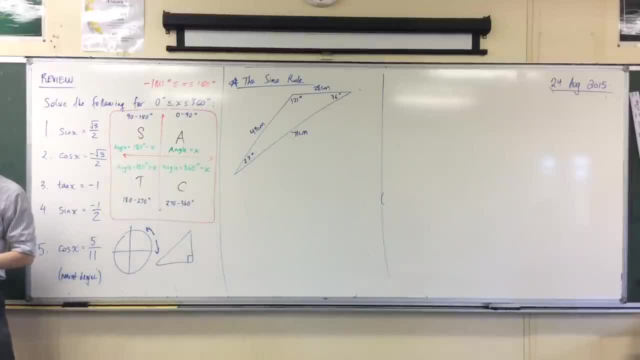 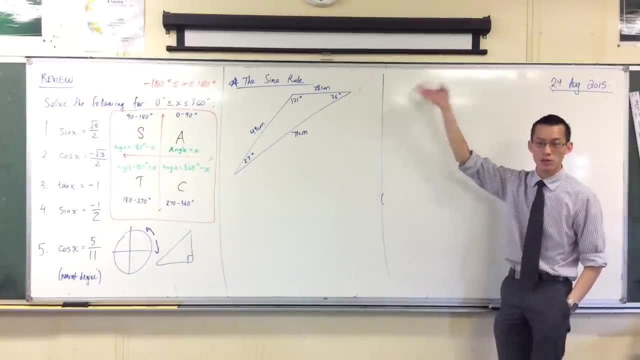 Hands up. Yeah, cool, All right, that's enough, Let's move on. If you're still going, that's okay. Just listen as you're doing that. What you should have is something that looks roughly like this: Okay. 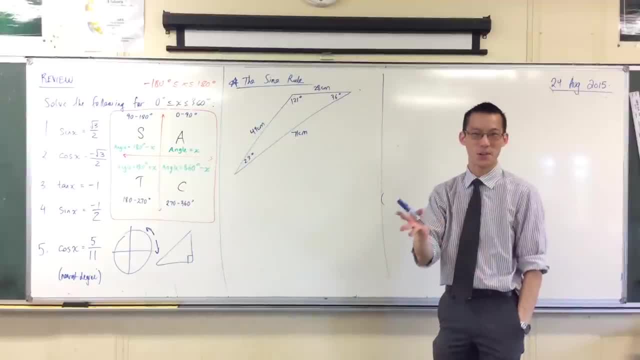 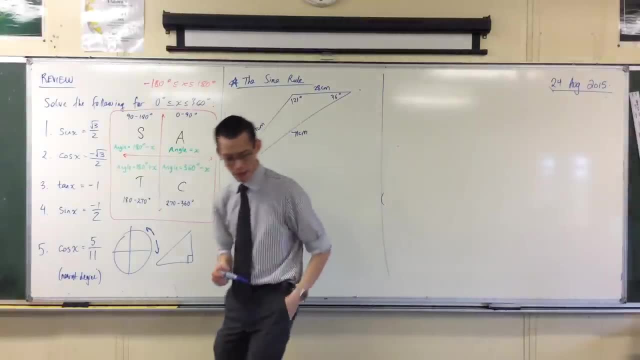 Well, actually I take that back. Yours will look nothing like this, probably because I've asked you all to draw different triangles, But the feature I'm about to point out to you on my triangle is Okay, out to you on my triangle you should be able to point out on yours. You can see, probably 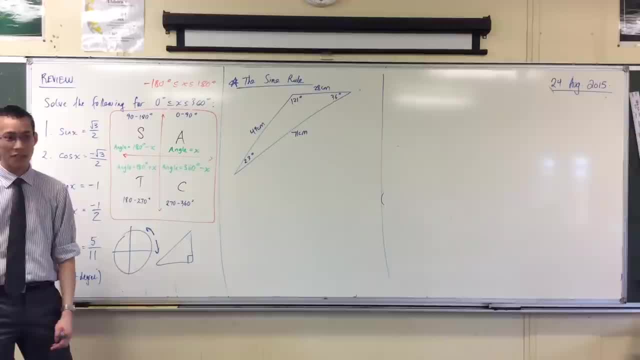 on most of you. one of your angles is bigger than the other two, So you have a biggest angle. If you've got an isosceles triangle or an equilateral one, you might not see that. Now mine you can see is 121 degrees. There's my biggest angle. Now I want you to pay attention. 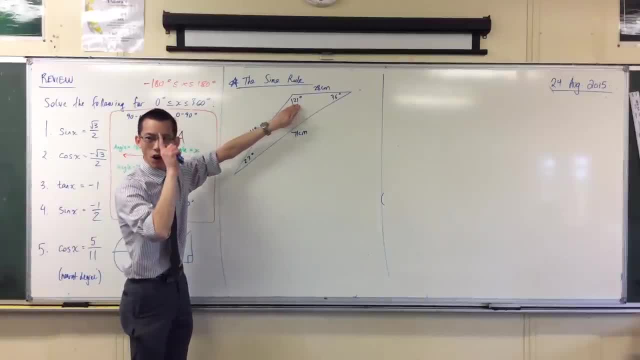 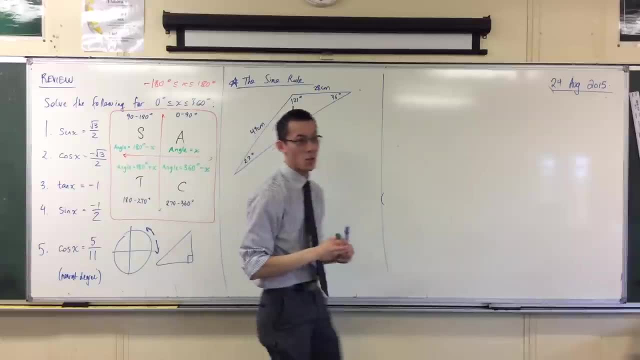 to the fact that this biggest angle is opposite the biggest side in the triangle. Do you see that? 121 degrees, That's opposite 71 in my triangle, which is clearly the longest side. And if you have a look at yours, look at the biggest angle and look at the side. 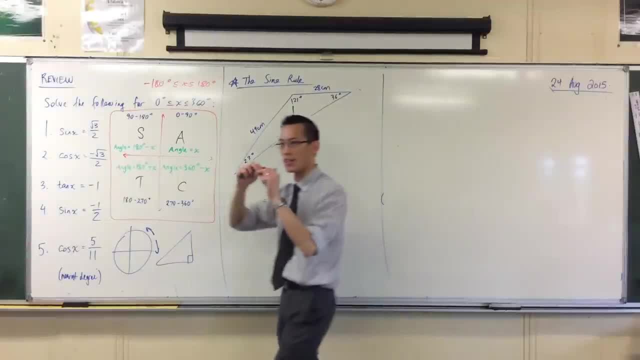 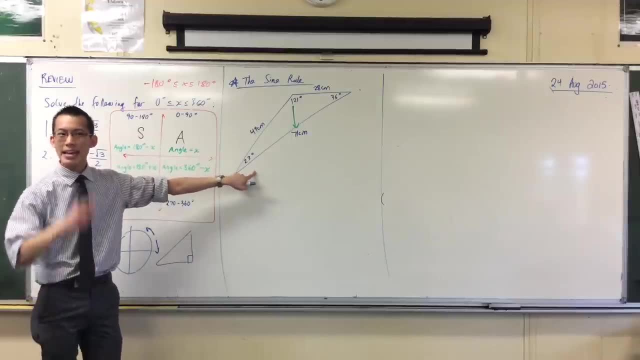 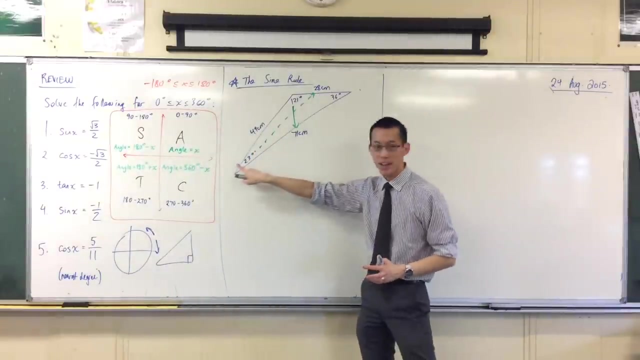 that's opposite it, facing it, and it should also have been the side that you measured out was the longest. Correspondingly, if you have a look at the smallest angle, it should also be opposite the smallest side, The smallest side and the smallest angle will be opposite. 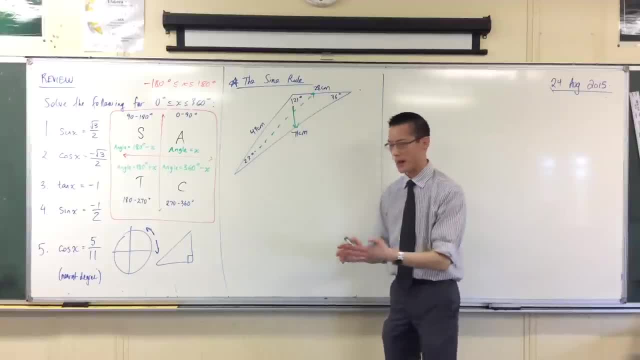 each other This way? right? Because if you think about it, if you just have a pair of random sides, a pair of random sides, and you take this angle in here between them, what we call the included angle, right, If you were to take those two and widen them, increase the angle? 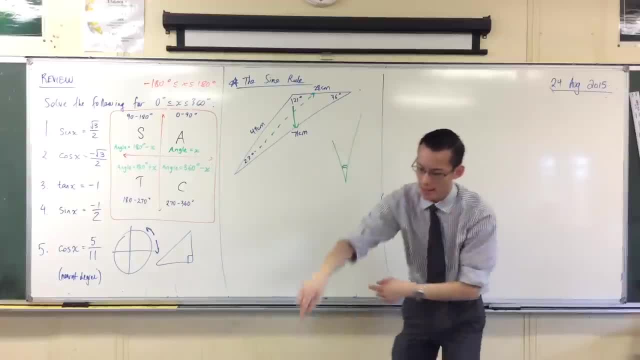 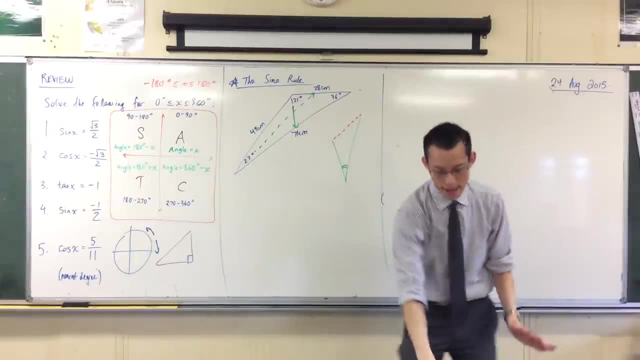 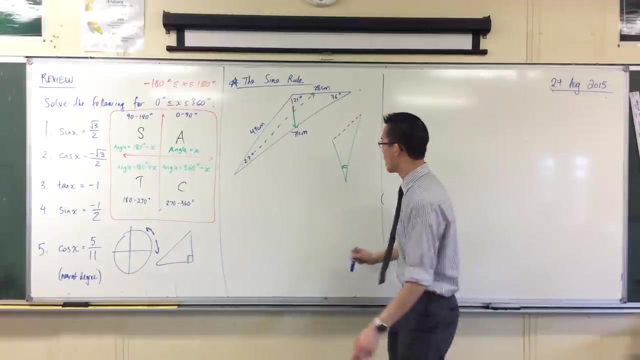 between them, you're necessarily increasing the length of the side that joins them, right? Do you see that This red length over here will get bigger and bigger and bigger as the angle that defines it gets wider and wider and wider. Okay, so let's just quickly jot this down, right? And, by the way, if you've noticed, 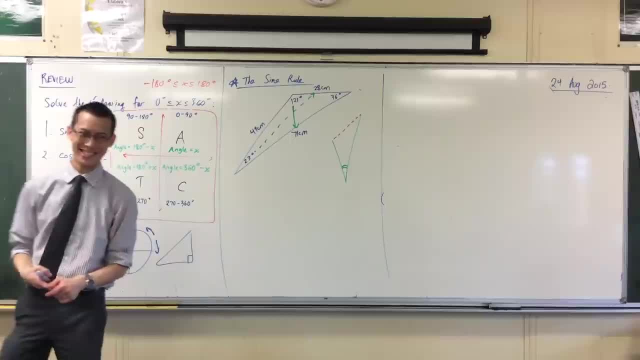 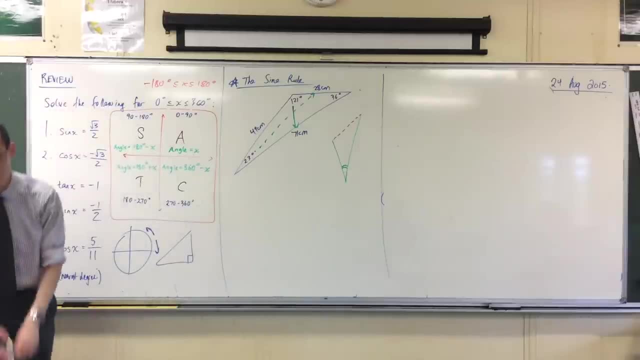 for example, those of you who created an equilateral triangle by accident- okay, because all your angles are equal, you've made all your sides equal as well. Or if you made an isosceles triangle by accident, if you've got two equal angles, then those are clearly not equal. 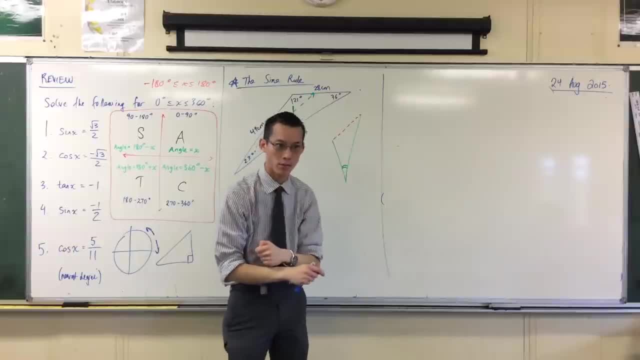 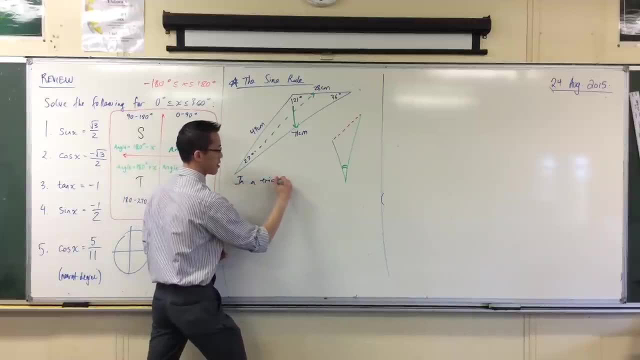 If you have two equal angles, then the sides opposite them are also equal right. There's a clear relationship going on here. Let's write this down right: In a triangle there's two angles. We started with the longest side. The longest side is always opposite the largest. 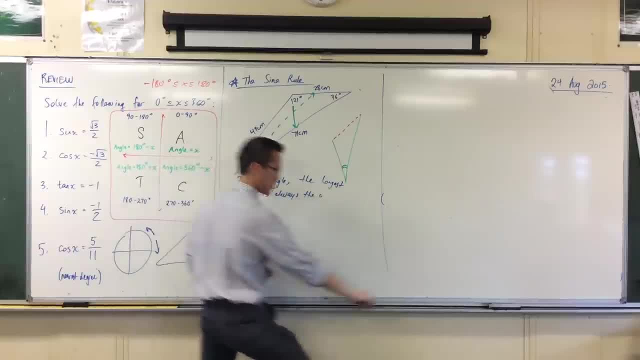 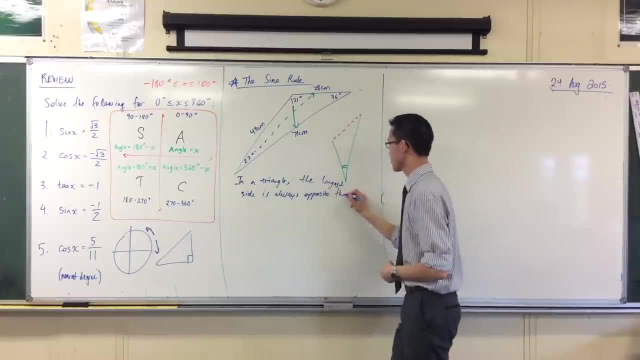 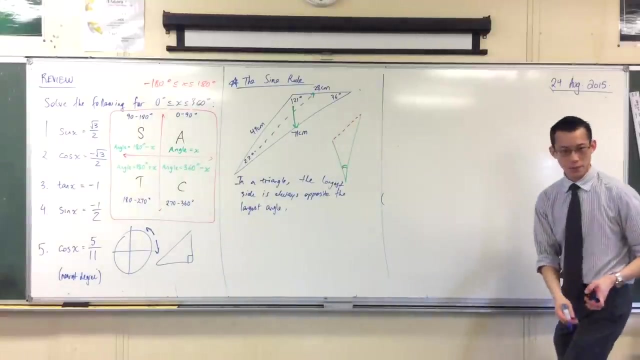 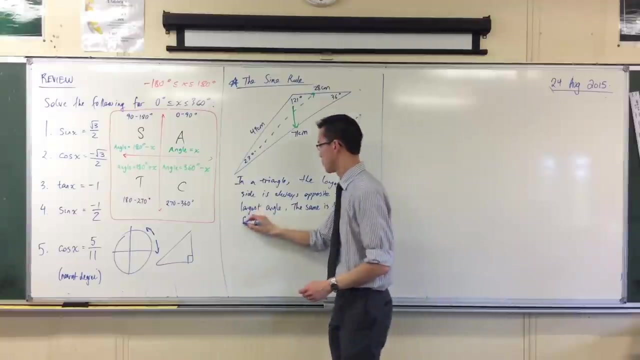 angle In a triangle, the longest side is always opposite the largest angle. The same is true for the side opposite the largest angle. In a triangle, the longest side is the smallest side, And if it's true for the longest side and the shortest side, it must. 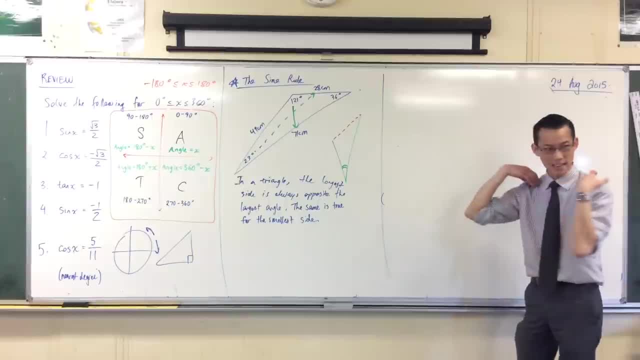 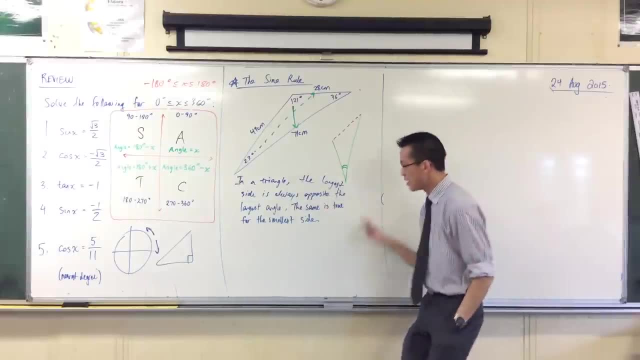 be true for the side that's left over right, And you can take the same pattern. if angles are equal, the sides that are opposite them are also equal. So this kind of thing seems like cannon fodder for understanding and using the trigonometric ratios to understand what's. 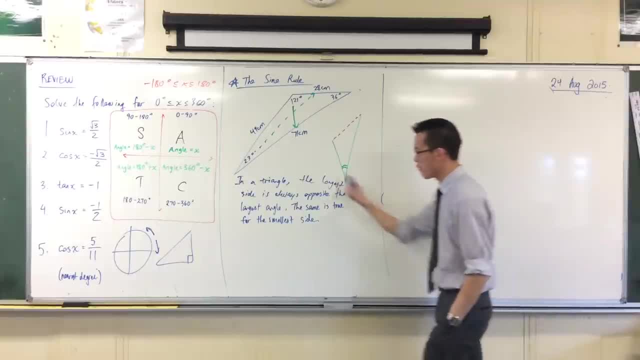 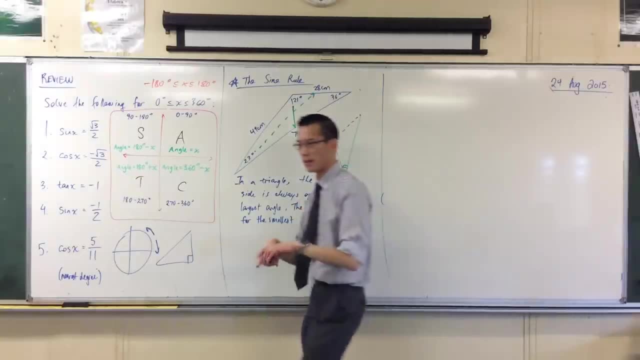 going on. okay, Now we want to use trigonometry to try to formalize this relationship. okay, But the problem with doing that is that in our triangle, all the triangles you've drawn, unless you've done this, coincidentally, none of them are.